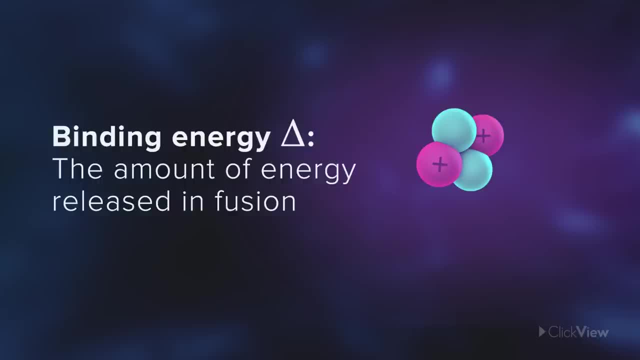 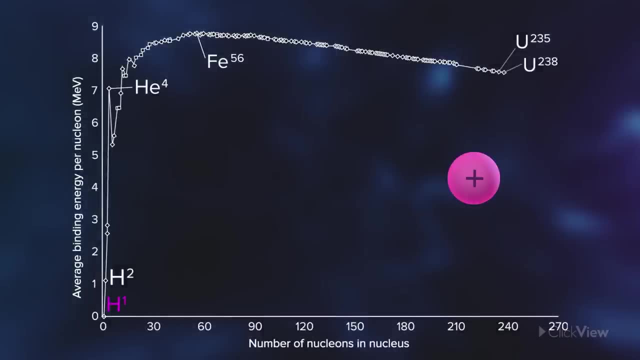 is called an atom's binding energy. Different elements have different amounts of binding energy and we can compare them on a graph. A single proton on its own, as a form of hydrogen, has no binding energy As the isotope deuterium. 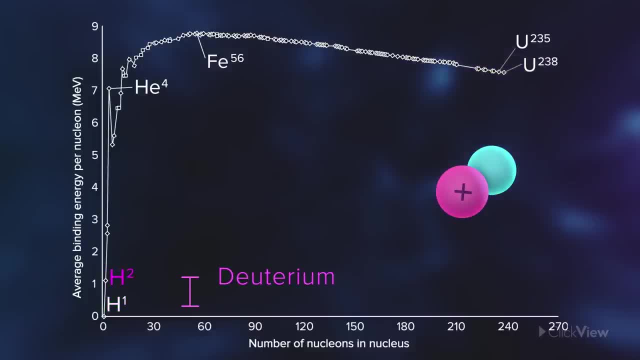 a proton and a neutron that underwent fusion would release a small amount of binding energy. Added to another deuterium nucleus to make helium, a much larger amount of energy would be released. As elements get heavier. differences in binding energy become smaller Beyond iron atoms. 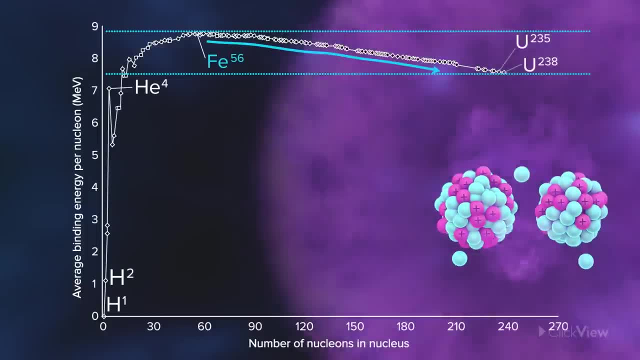 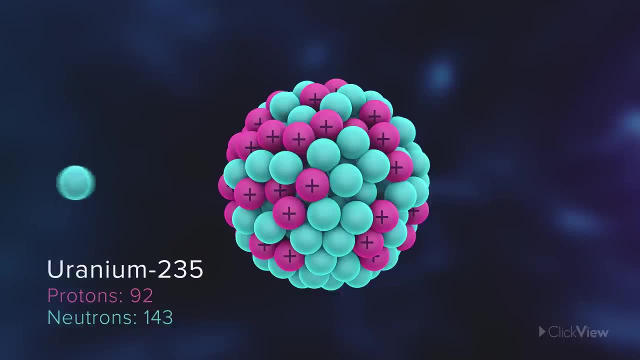 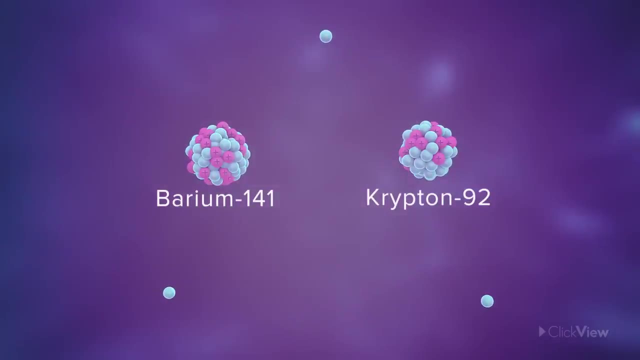 get so heavy, they release energy not as they grow, but as they break apart. When uranium undergoes fission to turn into an element like barium, it releases a tiny bit of energy. This is far less than the energy released as hydrogen combines into helium. 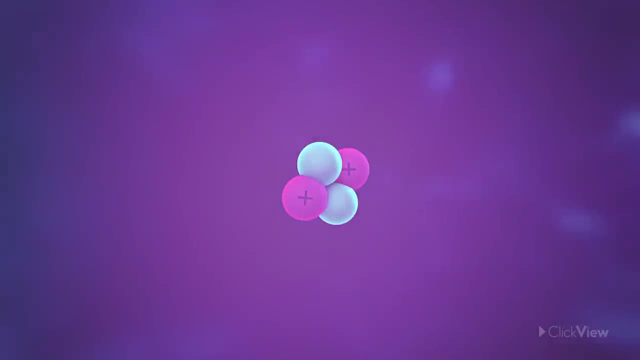 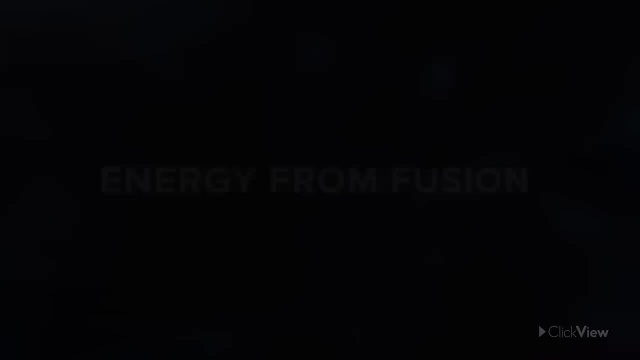 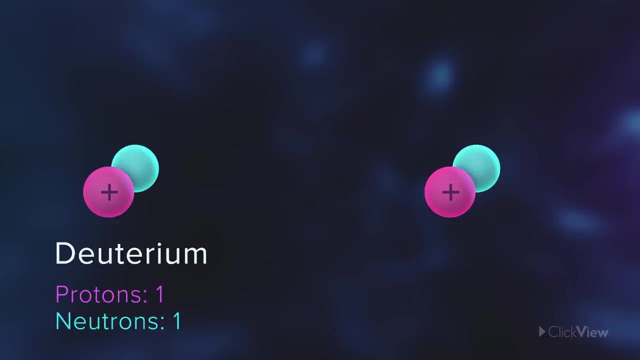 This makes the fusion of small elements a far more impressive potential source of energy than the fission of big ones. Let's see just how much energy. Instead of combining two deuterium particles, a more practical process involves sticking together a deuterium and another hydrogen isotope called tritium, which has two neutrons. 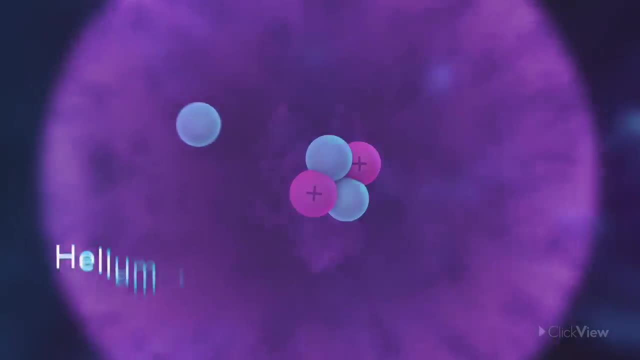 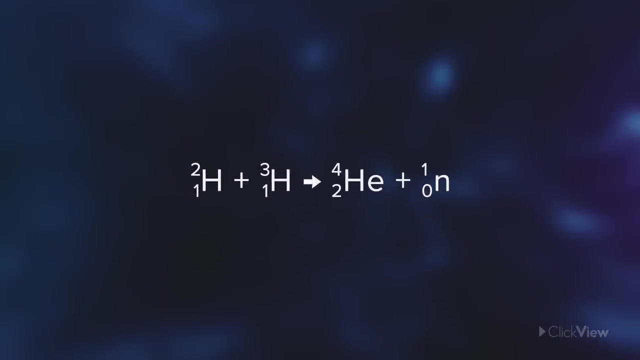 instead of one. The product is a helium nucleus and a single spare neutron. The mass of a single atom of deuterium can be rounded off to about 3.345 x 10 to the negative 27 kilograms. The mass of the tritium is about 5.01 x 10 to the minus 27 kilograms. 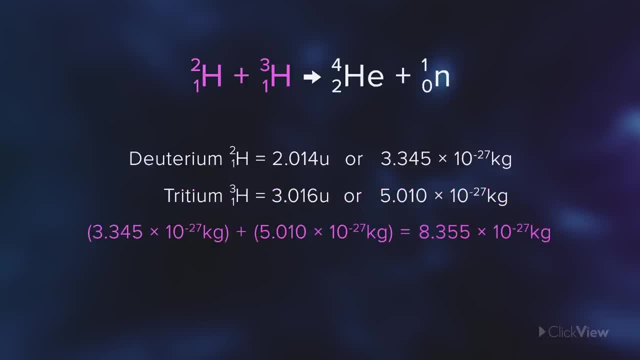 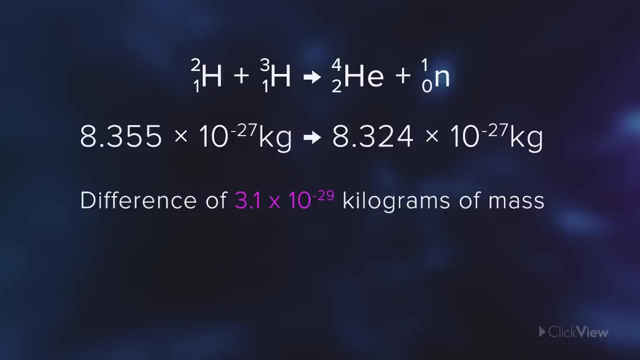 Both masses add up to 8.355 times 10 to the minus 27 kilograms, But in the form of helium plus a free neutron, the total mass is just 8.324 times 10 to the negative 27 kilograms. A tiny 3.1 times 10 to the negative 29 kilograms of mass seems to vanish. 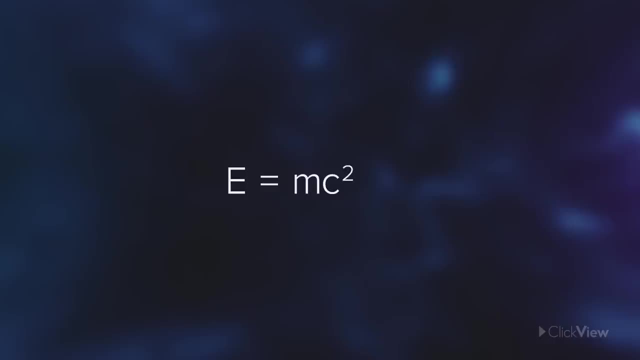 Remember Einstein's famous equation: Energy equals mass times, a super huge number: the speed of light squared. If we mixed 2 kilograms of deuterium with 3 of tritium, roughly 20 grams of mass would become other forms of energy. 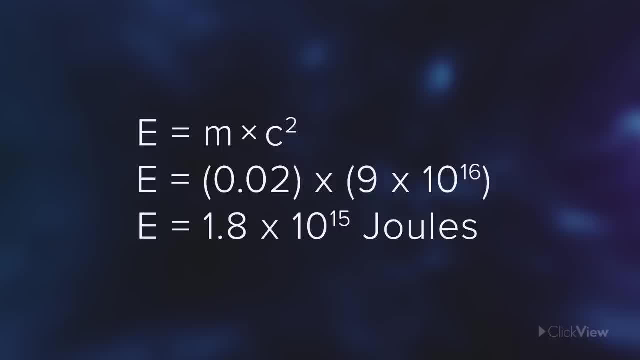 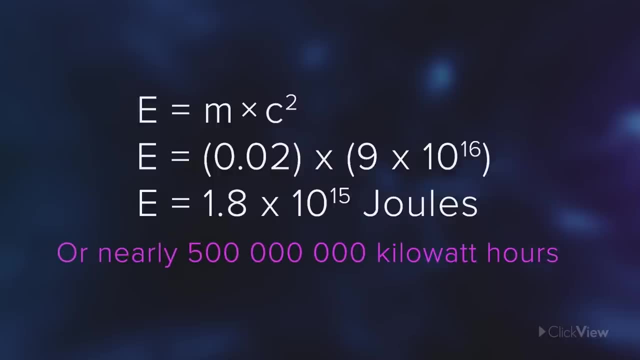 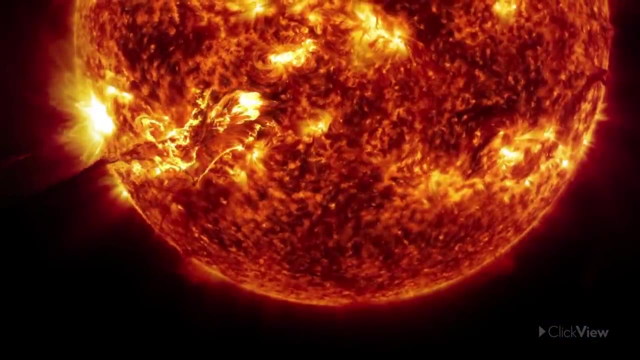 The difference between the reactants and the products would release 1.8 times 10 to the power of 15 joules as heat. That's enough to power about 50,000 homes for a year. Unfortunately, unlocking any of it requires technology. 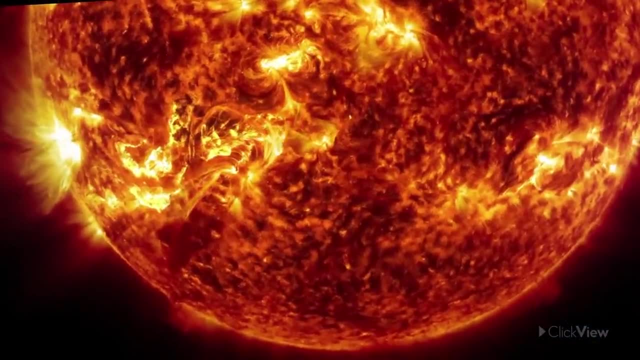 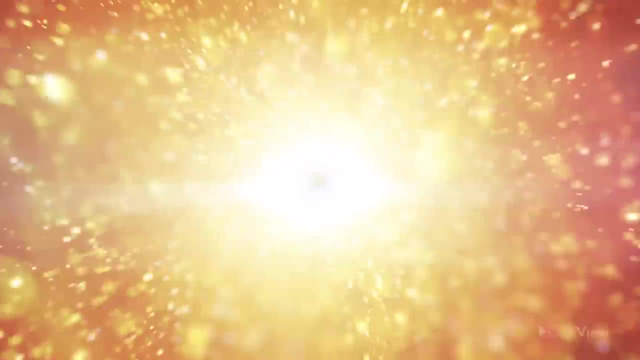 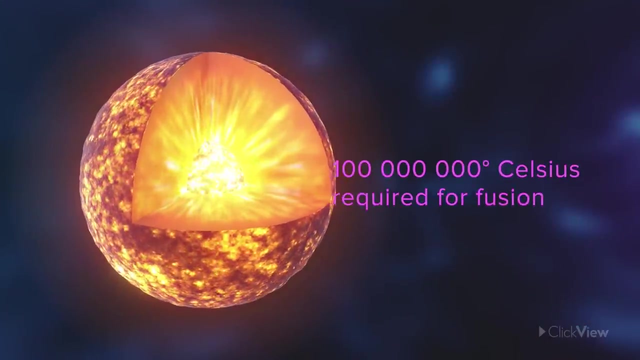 that can mimic the processes at work inside stars. Usually, intense gravity would provide the energy needed to force nucleons together. The good news is we can do the same job on Earth using heat. The bad news: The temperature required is over 100 million degrees Celsius. 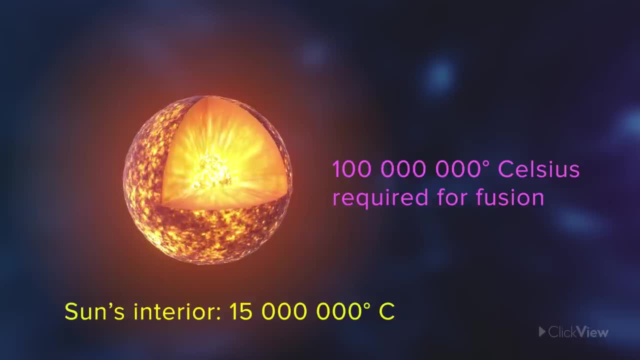 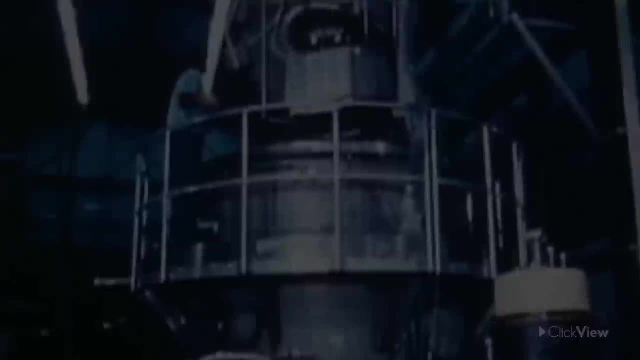 That's about seven times hotter than the interior of the sun. That's about 10 times hotter than the interior of the sun. That's about 10 times hotter than the interior of the sun. That's about 10 times hotter than the interior of the sun. 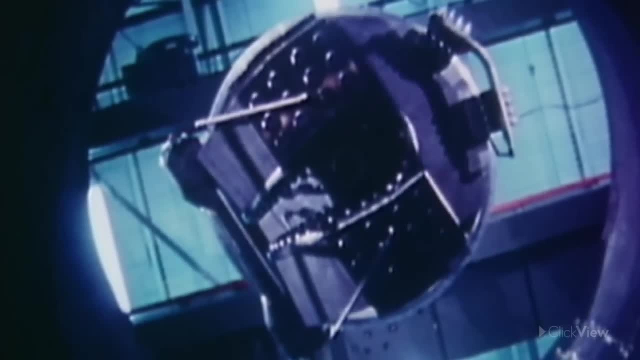 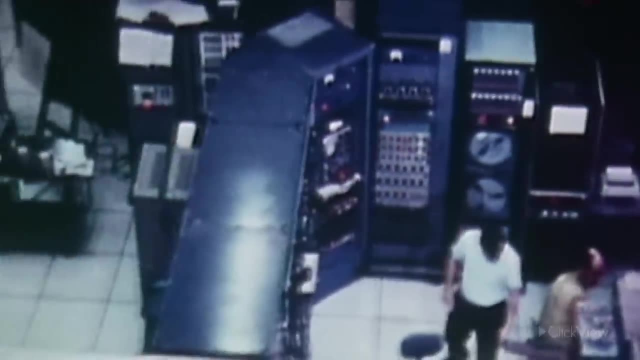 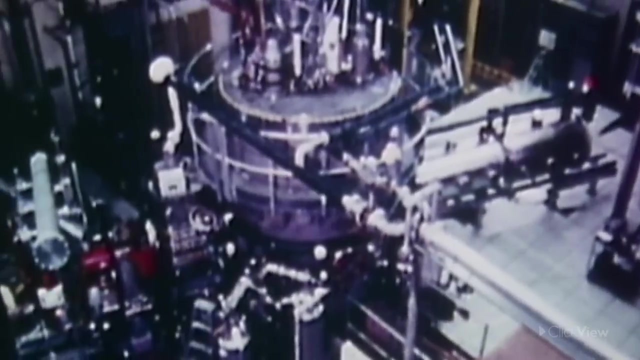 Nuclear fusion was conceived as a possible energy source in the 1930s. Since then, researchers have investigated a number of approaches for heating a gas made of small elements such as deuterium, to the point they sustainably undergo fusion. Two of the most promising forms of technology involve heating up a ring of gas called a plasma. 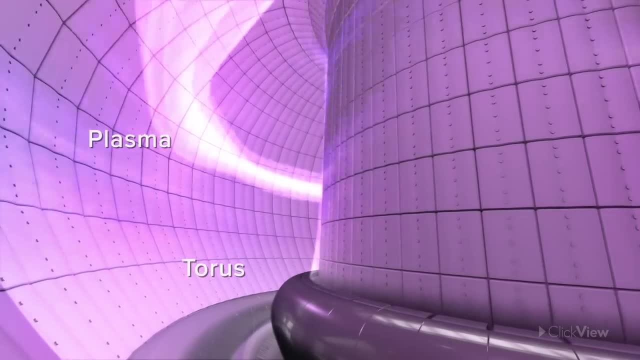 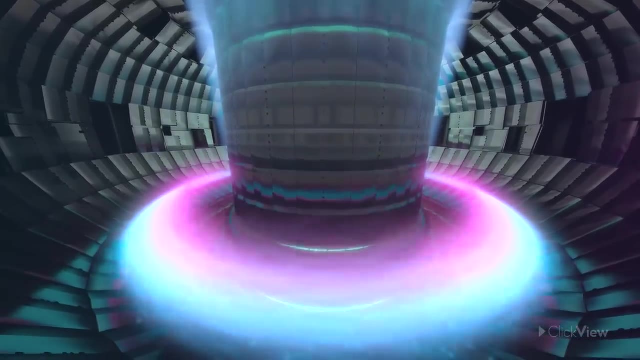 Two of the most promising forms of technology involve heating up a ring of gas called a plasma inside a doughnut-shaped tube called a torus. Plasma isn't exactly easy to control. Not only does it squirm like a ring of jelly, but its super-hot charged particles will quickly cool once they touch any surface. 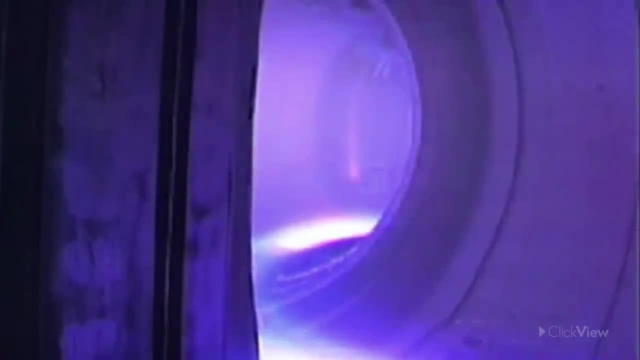 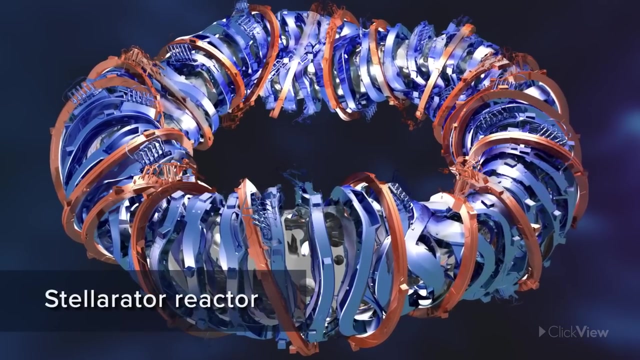 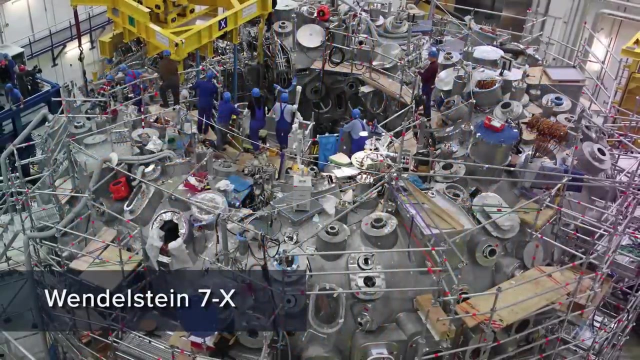 To keep the plasma hovering in place. two types of reactor use magnetic fields. Accelerator reactors use banks of magnetic coils to manage this task. Germany's Wendelstein 7X is leading the way in research on this form of fusion reactor. Its magnetic coils make the plasma easier to control.